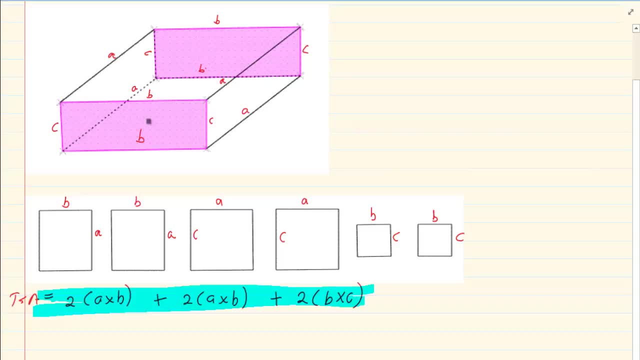 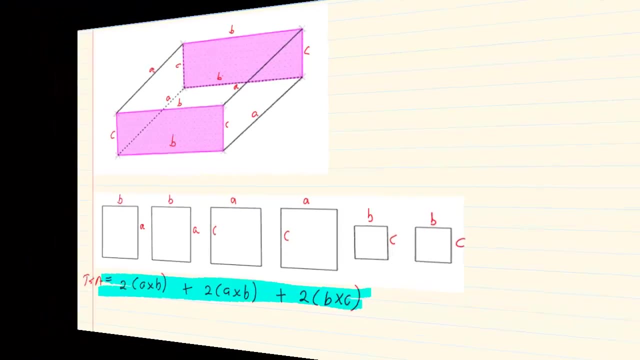 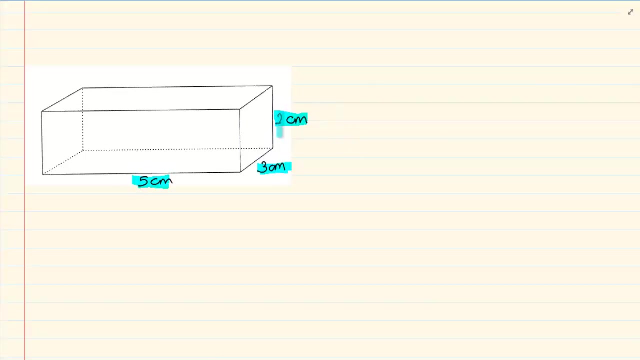 base. So when you are doing these questions, you need to know the difference: if it is a square base or if it is a rectangular base. Okay, now, when you look at the question, if you see that all the values are different, you can clearly see that this question is a rectangular base. 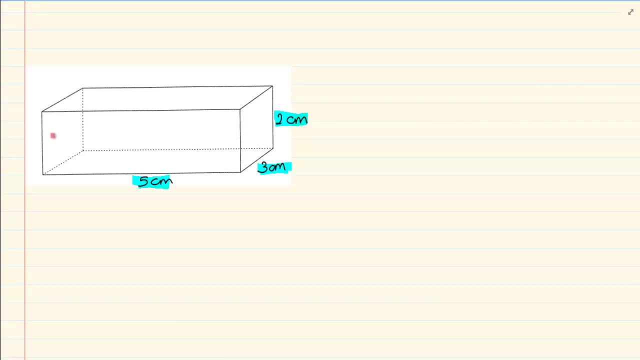 This side and the following side on the right and the left, which are the bases of the rectangular prism. This is a rectangular base. If you take the following one, can you see this one has a square base. So look at your formulas and then know which formula to use Now, when we have a rectangular. 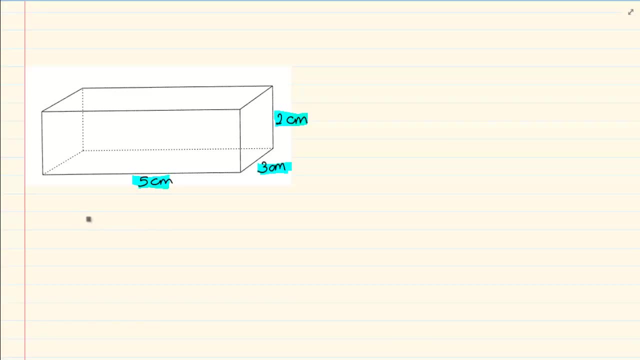 base. then we know we have the following formula: The surface area is going to equal to 2 times length, times breadth of the first shape. So let us work with the front and the back. Now, if you take that this side is 2, then remember the side opposite is also 2.. So it 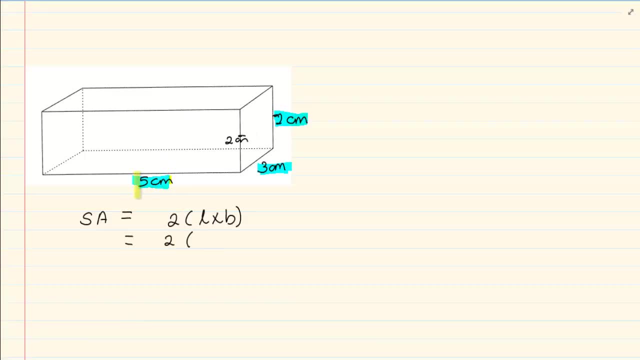 would be 2 into 5 times 2.. Then we would have had, plus again, 2 length times breadth, Because it is not a square base. we know that, it is not 4.. Now, what are we going to work out? Now we work the front and the back. 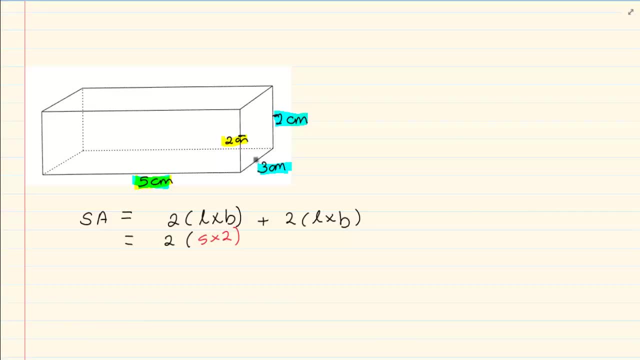 Let us work the top and the bottom. If this is 3, then immediately we know the side is also 3.. If this is 5, then the top is also 5.. So what is the area going to be? 3 times 5? and we know there is 2 of them. So we are going to have plus 2, 3 times 5.. Remember, it is the top and the bottom. 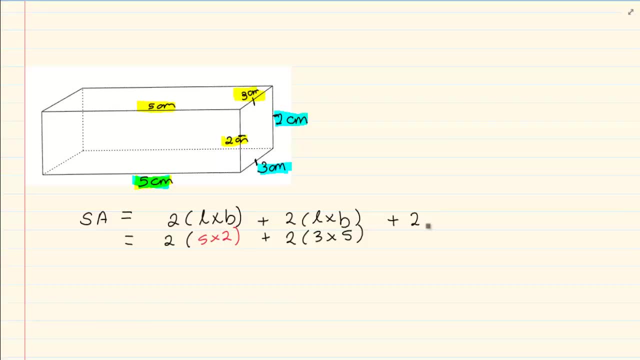 the bottom, Then we are doing the last one. It will be the one on the right and the one on the left. Now what is the area of that specific shape? It will also be 2 times length times breadth, and if we look at the values, it is 2, 3 times 2.. Now, from here you can. 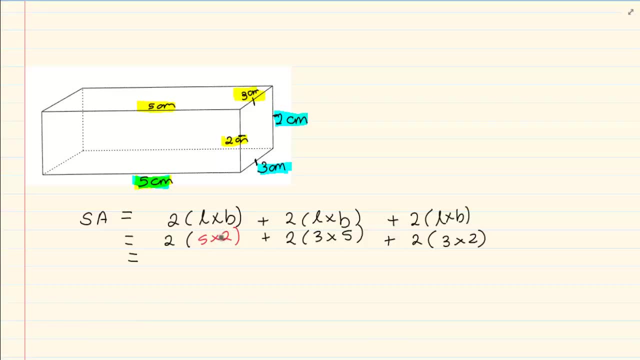 use your calculator, but it is easier to just do the values We know. 5 times 2 is 10, 2 times 10 is 20, plus 5 times 3 is 15, times 2 is 30.. 3 times 2 is 6, times 2 is 12.. So 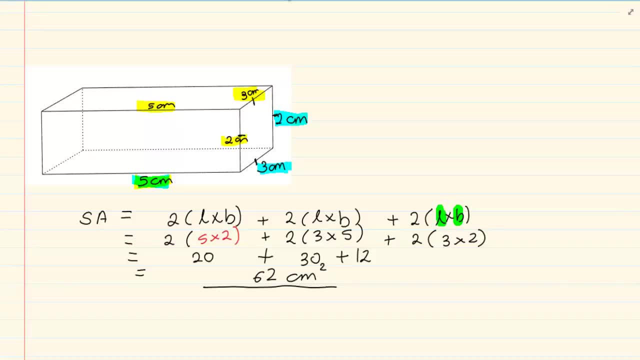 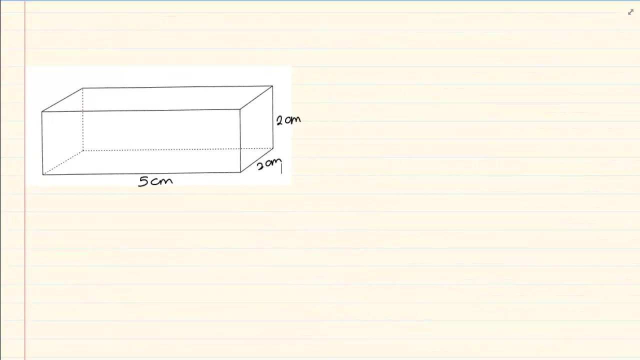 our final total is 62.. Now it is going to be cm2.. Why cm2?? We are working with area. we are multiplying 2 dimensions: length times breadth. So let us do one that has a square base. Let us look at the following rectangular prism. What you notice is that the base, which 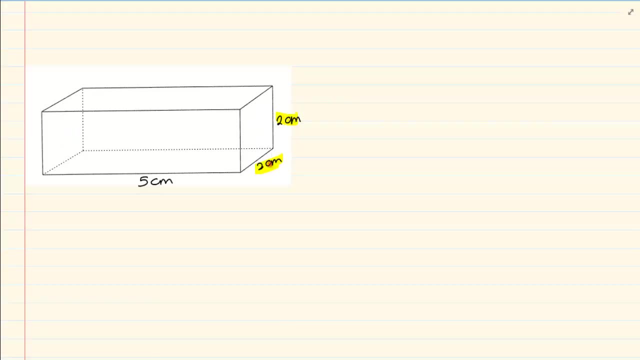 means the side on the right and the left is a square. Both are 2 cm, So when we are using a square base, then we know we are going to have 2 length times breadth plus 4 length times breadth. Now, we had discussed this type of surface area in our previous videos. This: 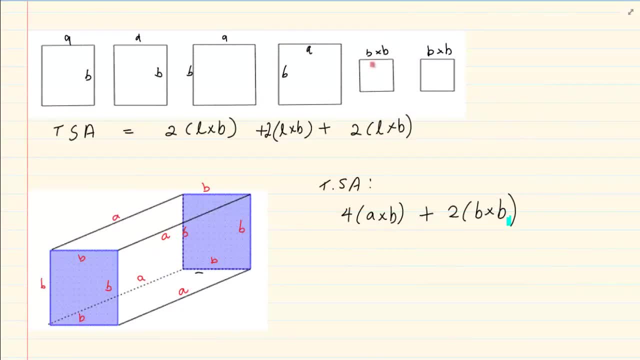 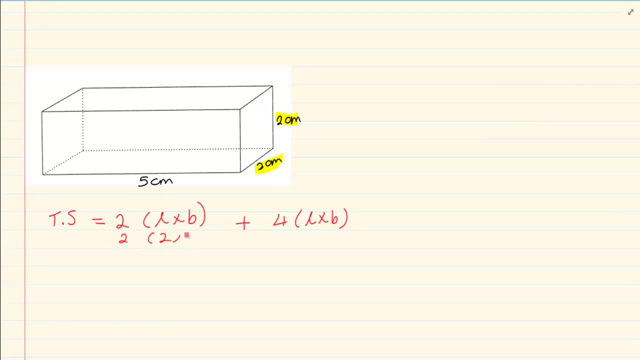 is where we had discussed that the bases are squares. So if we take the base, it would be 2 into 2 times 2. Then we have got plus 4.. Now if this is 2, then we know the top is 2. 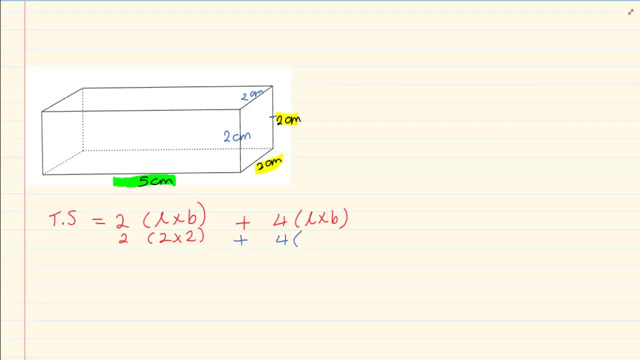 and we know that a cross is also 2.. So what are the values? we are looking for? The 5 and the 2.. So we have 4 into 5 times 2.. 2 times 2 is 4, times 2 is 8, plus 5 times 2 is 10.. 10 times 4 is 40. So the total surface. 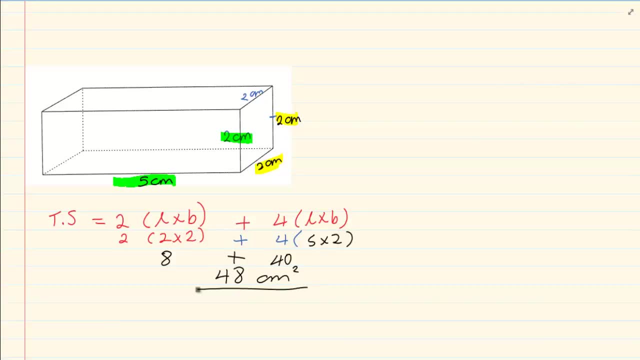 area is 48, but you are going to put cm2.. Remember, area is squared. Thank you for watching.